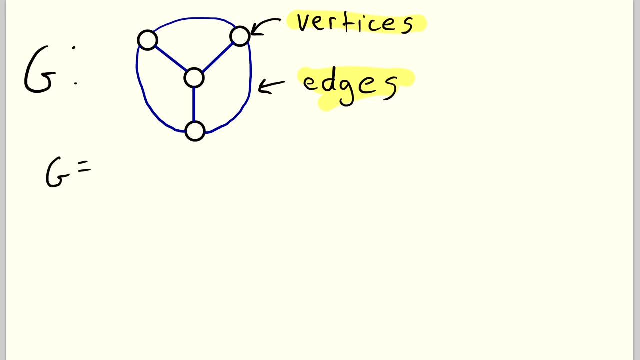 Well, a graph that we'll call G, of course, is an ordered pair with some vertex set that we'll call V, And, like I said, it's an ordered pair, So it's important that the vertex set comes first and then the edge set comes second. 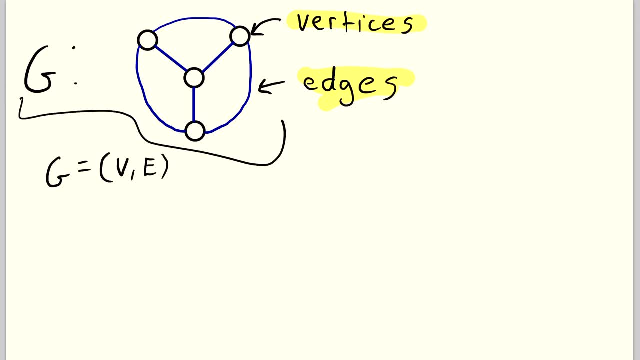 So if we wanted to write out this graph up here in this way, how would we do it? Well, right now we can't, because we haven't labeled the vertices or edges in this graph. It's currently unlabeled, So without any names to put to the vertices or edges. we can't write it out explicitly, with all of its vertices and edges in this form. 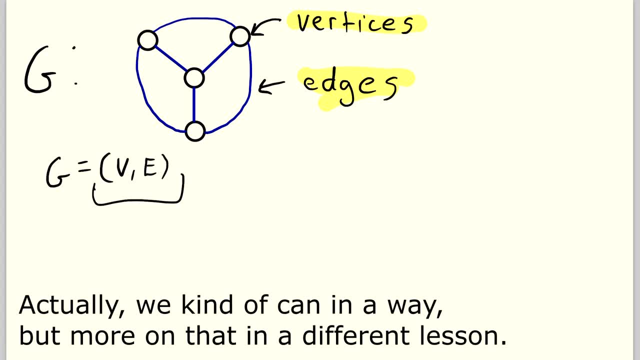 So without any names to put to the vertices or edges. we can't write it out explicitly with all of its vertices and edges in this form, And sometimes this is fine. Sometimes all we want is this visual representation of a graph, And that's really what you want. to look at the graph's structure. 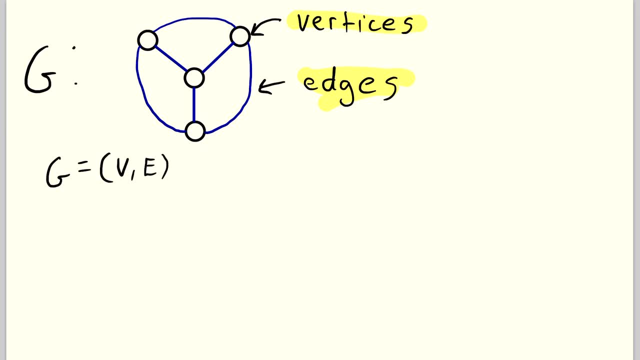 But for the sake of this lesson we're going to throw some labels down, So we'll call this vertex 1,, this one 2, and this one 3, and this one 4.. Hope you can read those numbers, all right. 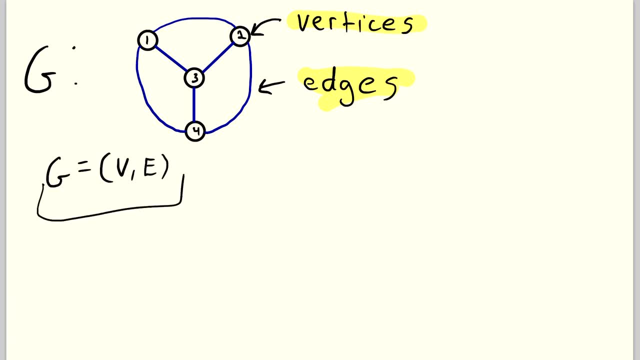 So then, if we want to write the graph out in this form, how do we do it? Well, I'm going to erase this so that we have some more room to write it out And let's start Again. it's an ordered pair, so we open up the ordered pair. 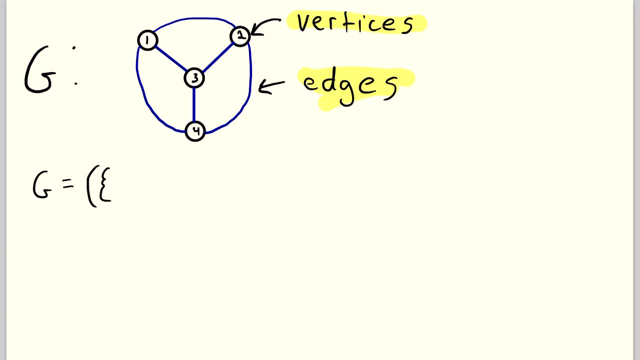 And then the vertex set comes first. so we open up the vertex set And what do we put in it? Well, of course we put in the vertices 1,, 2,, 3, and 4.. Those are the four vertices in the graph G. 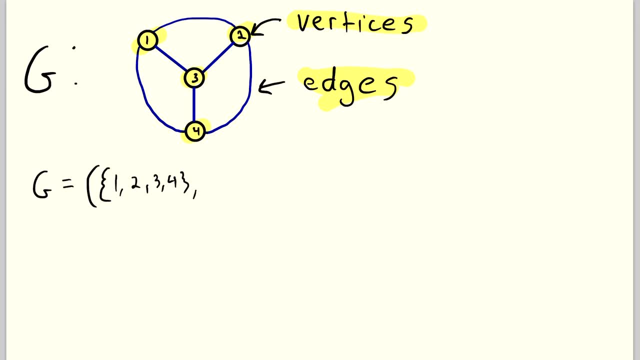 So those are the four objects that go in the vertex set. Then comes the edge set. The edge set is a little trickier. It's comprised of two element subsets of the vertex set. The two elements, The elements that go into each subset, are vertices that are joined by an edge. 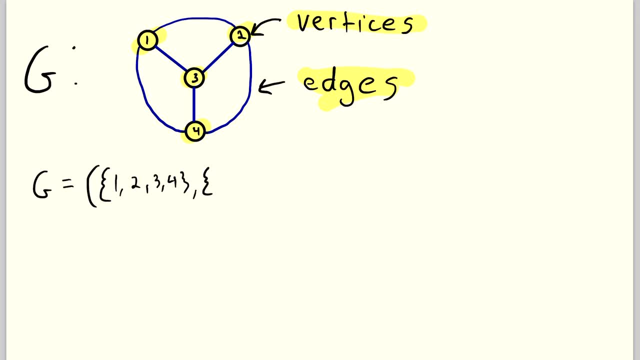 And I know that might be a little unclear. so let's just look at an example. Here we have an edge joining vertex 1 and 2. So to represent that in the edge set we write a set that has the vertices 1 and 2 in it. 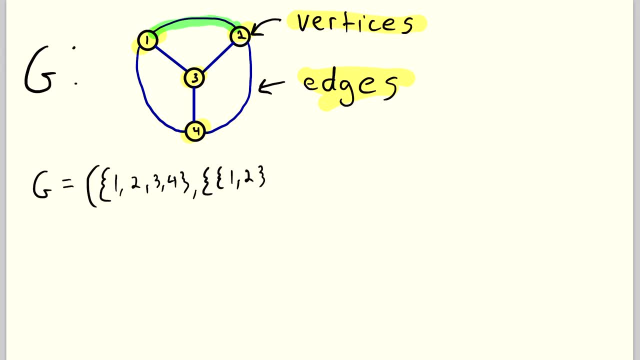 And that's all there is. You could also write it as the set containing 2, 1.. Remember that doesn't matter, because sets are not ordered. So then 2 is joined with 3.. So we also have to write the edge 2, 3 in there. 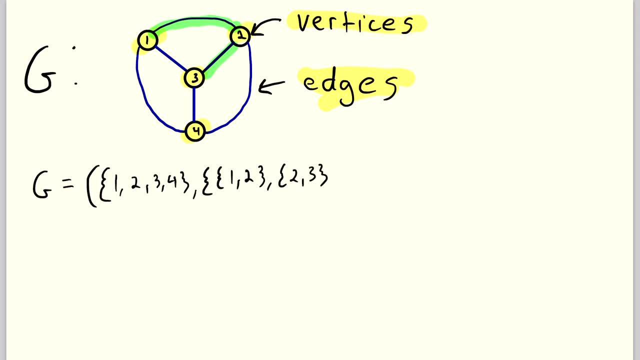 And again you could write it as 3, 2.. Doesn't matter. Order of the vertices doesn't matter. All that matters is that they're joined by an edge, And I'll go ahead and write the rest of these out. 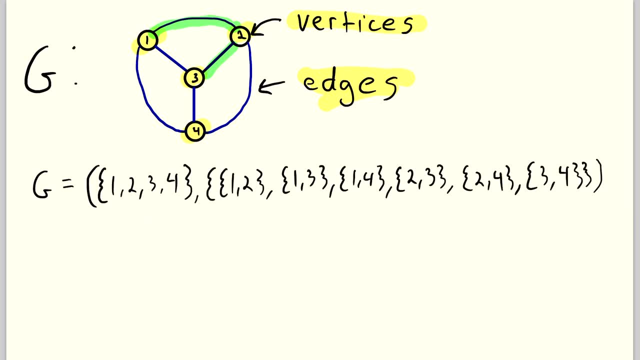 So here we go. This is the graph G written out explicitly as an ordered pair, with this vertex set and this edge set, And you can see all the edges here in the set. So we already went over 1, 2,, which is right there, and 2, 3,, which is right there. 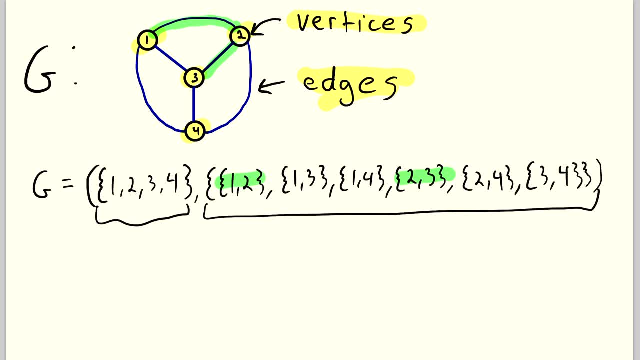 2, 3, which is right there, And we just rewrote it so that it would fit more nicely. And let's look at the other edges. 1 and 3 are joined by an edge. We see that represented there. 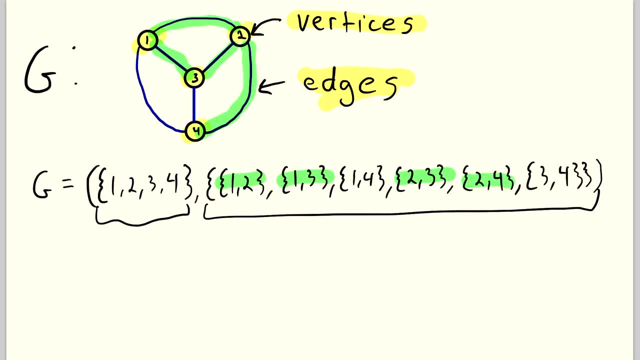 2 and 4 are joined by an edge. We see that represented there. 3 and 4, that's right there, And 1 and 4, right there. And I wrote all of these with the lower numbered vertex first and the higher numbered vertex second. 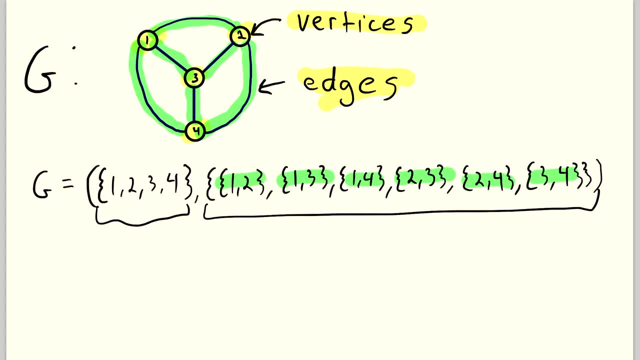 I just want to make sure it's absolutely clear. that is not important. You could write all of these edge sets in reverse order, So 2, 1, 3, 1, 4, 1, 3, 2.. 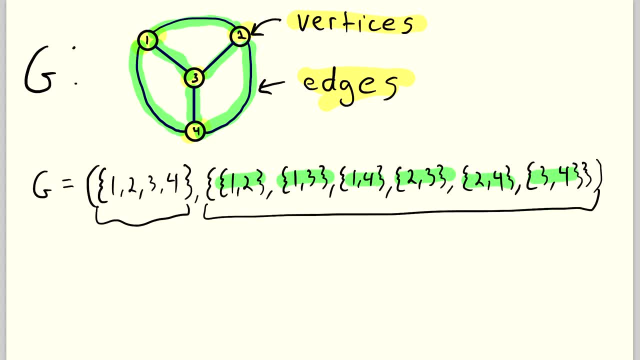 That does not matter Again. all that matters in the edge set is that the vertices you list in these subsets are joined by an edge, And I'll also mention that in this case, this graph G that we see here is an example of a complete graph. 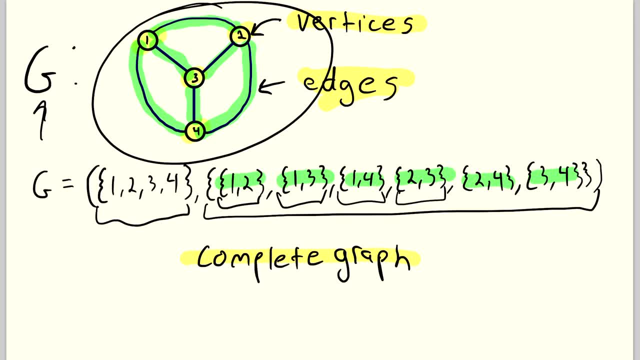 because every pair of vertices is joined by an edge. And if in a graph every pair of vertices is joined by an edge, we call it a complete graph. But I'll talk more about those in a different lesson. Now one other thing I want to touch on. 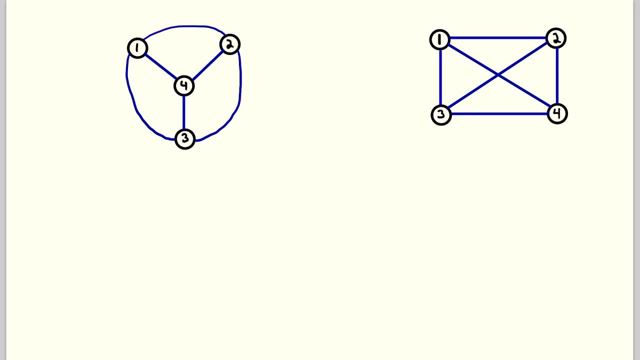 is the visual representations of a graph. So, like I said, a graph is an ordered pair with a vertex and an edge set. That's a formal definition of a graph, But we can also draw them like you see here, And let's name these graphs. 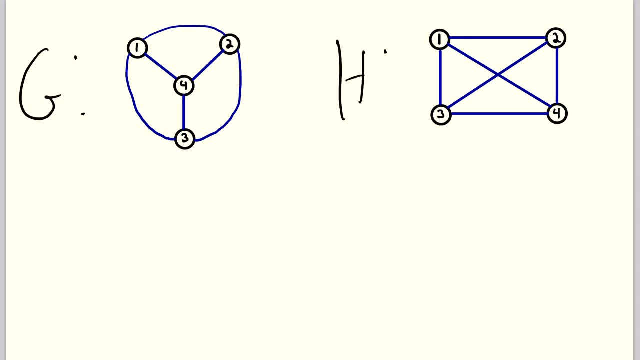 So this one is G and this one is whoops, that was a bad H, This one is H. The point I want to make here is that, while these graphs look different, this one is the one we just talked about and this one looks different. 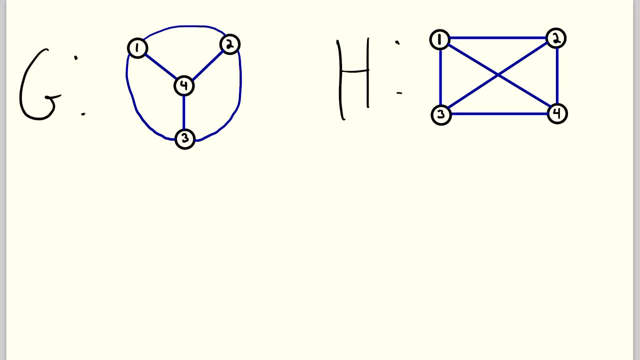 They are in fact the same graph. You can draw any graph in an infinite number of ways, But what's important is what vertices and edges it has. So two graphs are equal if they have the same vertex set and the same edge set. 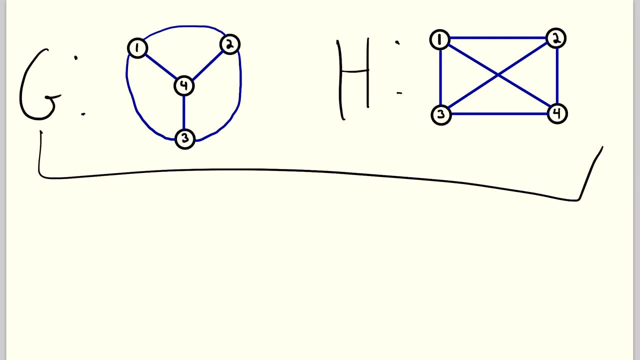 So are these graphs here equal? Indeed they are. And how do we know? Well, like I said, we know they're equal if they have the same vertex and edge sets. So let's go through it. Graph G has vertices 1,, 2,, 3, and 4.. 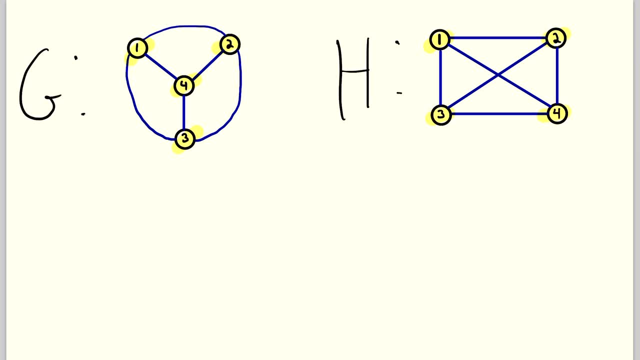 Graph H similarly has vertices 1,, 2,, 3, and 4.. Then we just have to look at the edges. 1 is joined with 2.. 1 is joined with 2.. 2 with 3.. 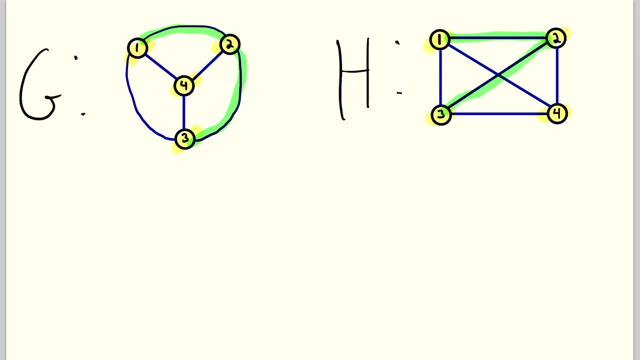 2 with 3.. Whoops, that was bad. 2 with 3.. 3 is joined with 4.. We see 3 is joined with 4 over there, 1 is joined with 4.. And 1 is joined with 4 over here. 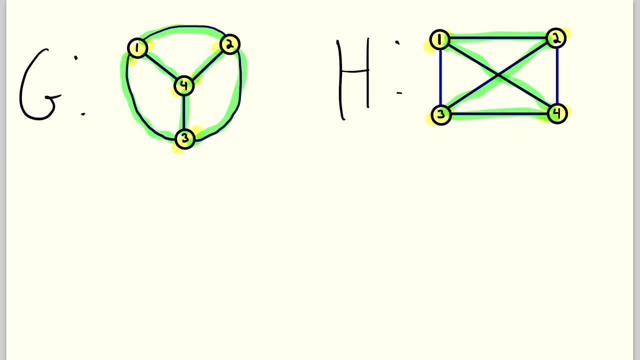 And then we have 2, 4, and 1, 3 in G, And we also have 2, 4, and 1, 3 in H. So we see clearly there that these graphs G and H have the same vertex and edge sets. 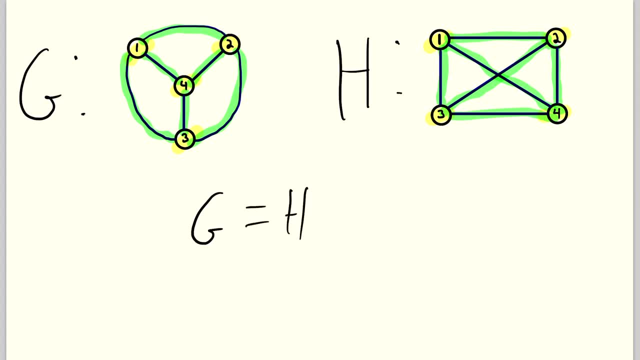 Thus we can say that G is equal to H. So again, you can draw graphs to look totally different when they might in fact be the same graph, Just as another example. let's say we had these two vertices, vertex 1 and 2.. 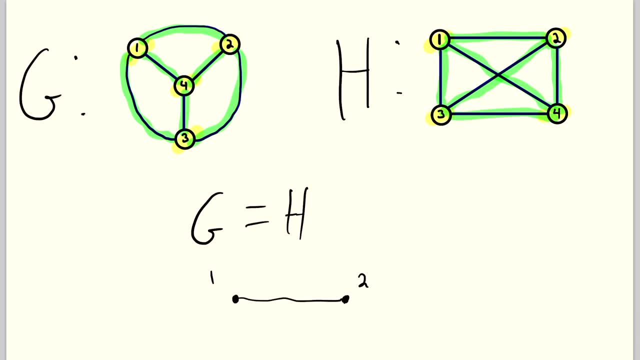 We could join them with an edge like that, And that's a fine graph. And that graph is indeed the same as this graph, where 1 and 2 are joined by this ridiculous edge. All that makes them equal is that they have the same vertex set. 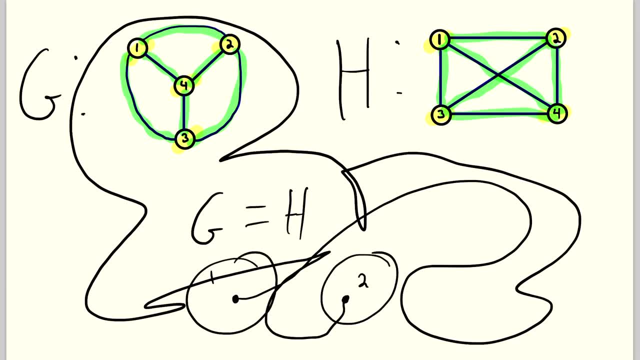 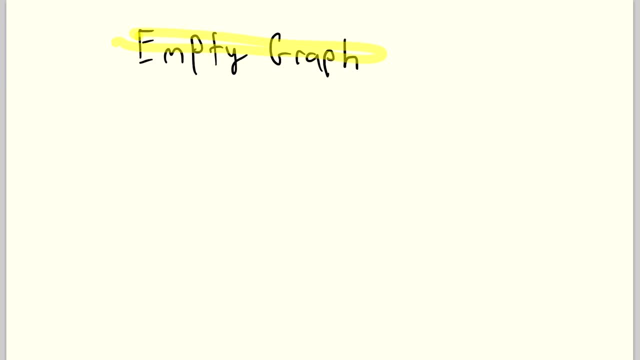 1 and 2, and the same edge set, namely an edge joining 1 and 2.. I know it looks like a mess, but I hope the point is clear. One other thing I want to talk about is the empty graph. 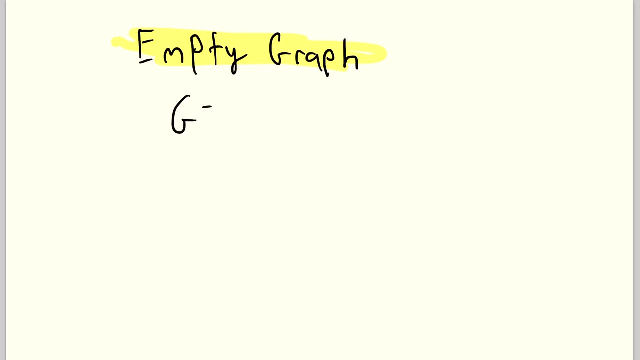 What is the empty graph? Well, an empty graph is any graph that has an empty edge set. So it's an ordered pair with some vertex set and an empty edge set. So a graph like this, or like this, or like this. 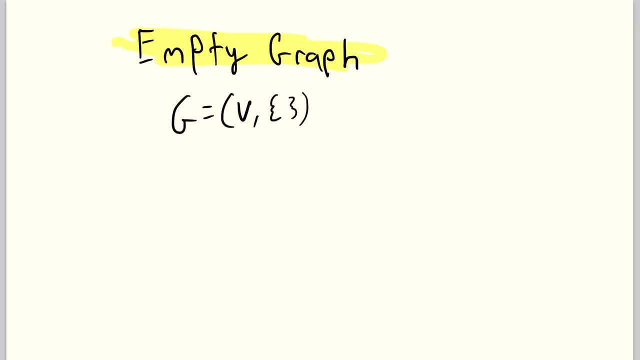 it has vertices but no edges. That is allowed, It's perfectly fine, And we call such graphs empty graphs. The only other sort of tricky bit is that if the graph has no vertices either, so if it has an empty vertex set and an empty edge set, 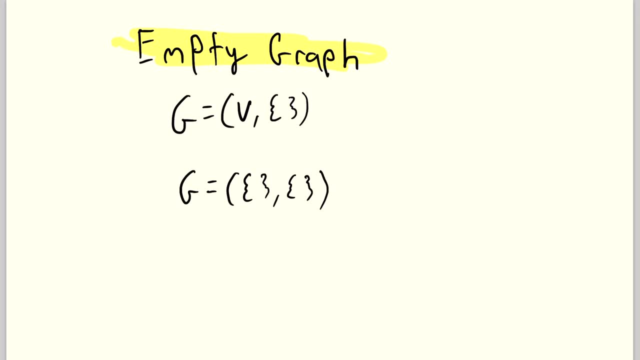 whoops, I don't know why. I wrote that extra comma. So an empty vertex set and an empty edge set. this is sometimes considered a graph and sometimes not. It depends on the author and the text. So just be aware that this could be considered a graph or not considered a graph. 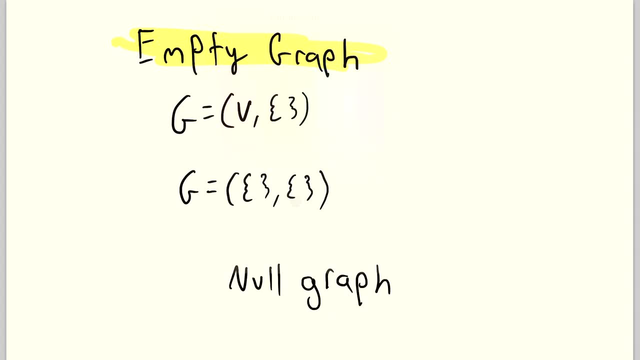 depending on what you're reading, If it is considered a graph, it's sometimes referred to specifically as the null graph, which is the empty graph, but with zero vertices. And then, lastly, let's just look at an example with some words. 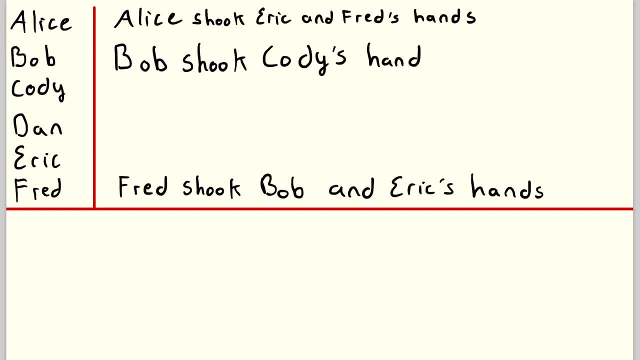 So this is an example of how a graph can represent objects and how the objects are related, And that's really what graphs are all about. So let's say, Alice, Bob, Cody, Dan, Eric and Fred- six intrepid heroes- are going to a hootenanny, a party, a fiesta. 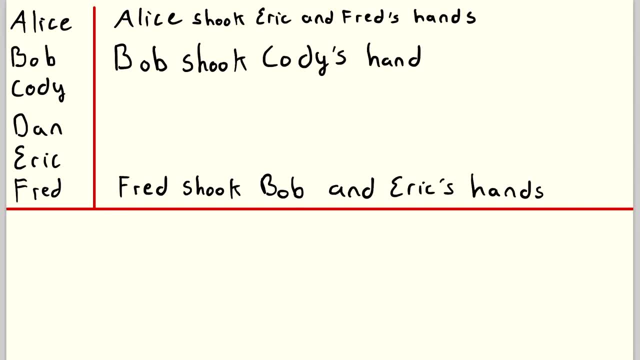 They're going to have a good time And at this most celebratory event, they are shaking hands And we want to write a graph, draw a graph that represents the people at the party and who has shaken hands. Well, we've got our objects over here. 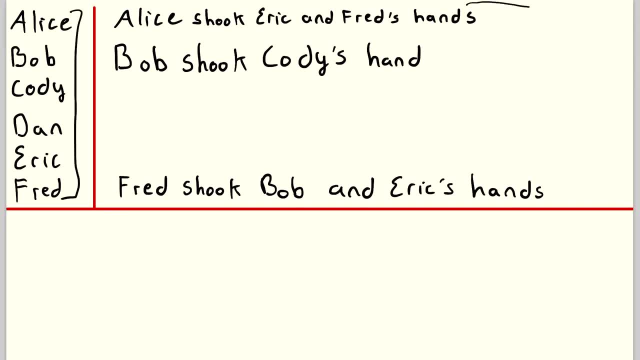 the names of the party goers, and we have their relations over here, which are the pairs of people who have shaken hands. So how are we going to draw our graph? Well, to begin with, we need the vertices, which represent all of the objects in this situation. 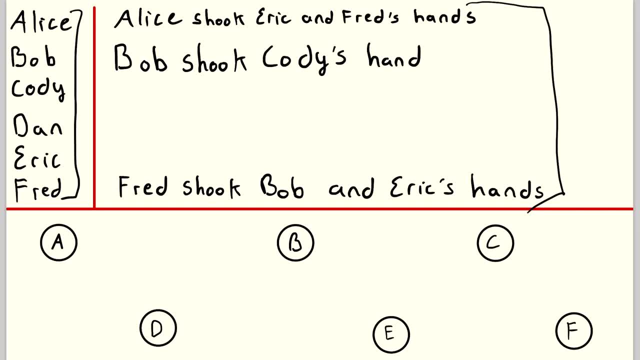 In particular, it represents the people. So I've labeled each vertex with the first letter of the party goers names. And now all that's left for the edges is to join the people who have shaken hands. So I'll write the edges in blue. 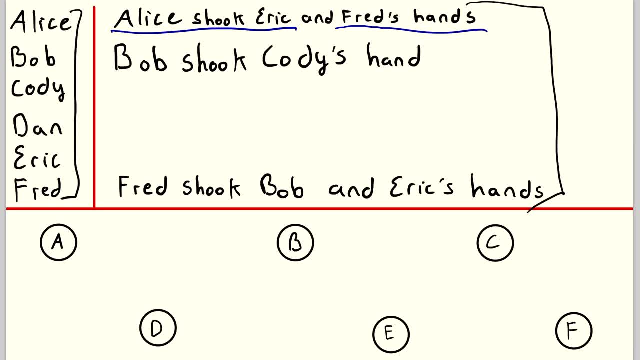 We see that Alice shook Eric and Fred's hands so we have to join A with the E vertex and with the F vertex. We see that Bob and Cody shook hands so we can join the Bob vertex with the Cody vertex and Fred shook Bob and Eric's hands. 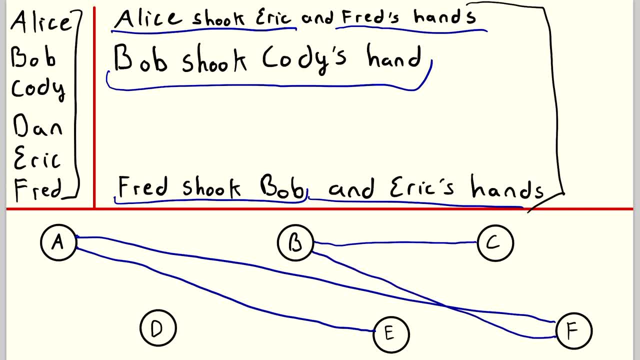 So we will join F with the B vertex and we will join F with the E vertex, And that's just an example of how easily we can use a graph to represent objects and how they relate to each other. It's a very classic, often used graph theory example.